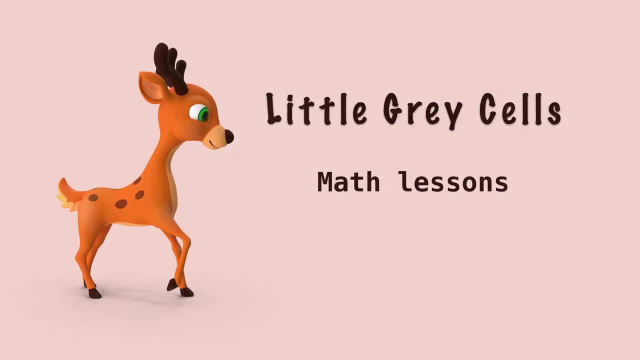 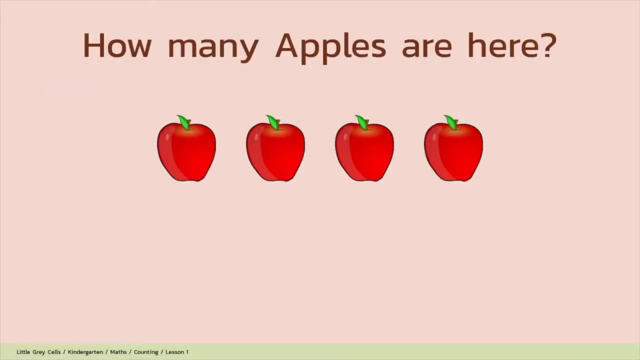 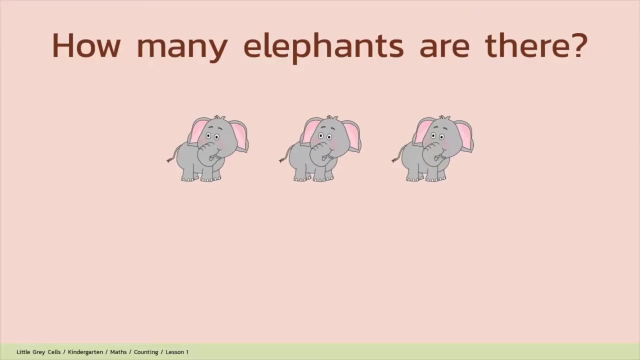 Little gray cells. Math lessons Counting up to 10.. How many apples are here? All right, shall we count 1,, 2,, 3,, 4.. The answer is 4.. Good job, How many elephants are there? 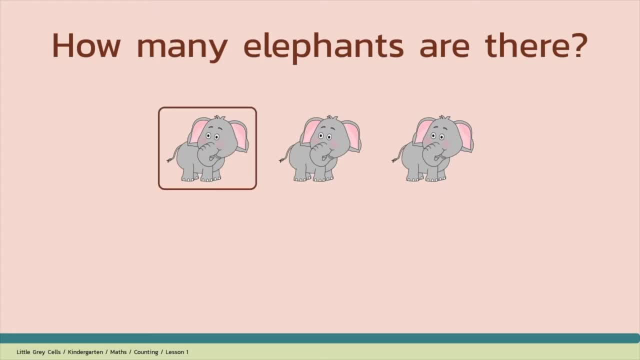 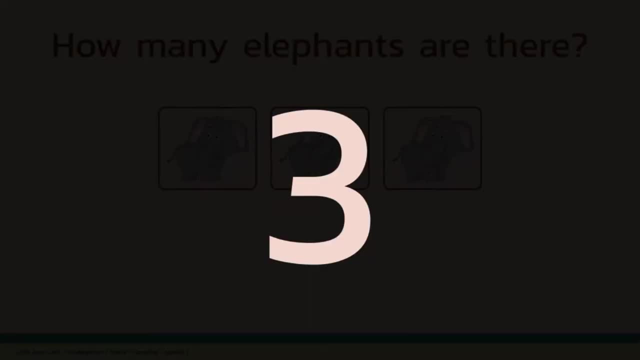 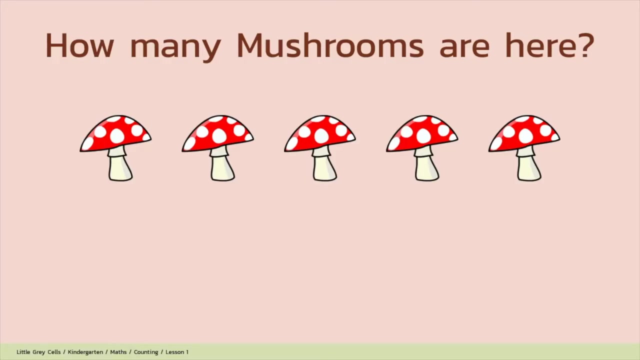 All right, shall we count 1,, 2,, 3.. The answer is 3.. Good job. How many mushrooms are here? All right, shall we count 1,, 2,, 3,, 4, 5.. 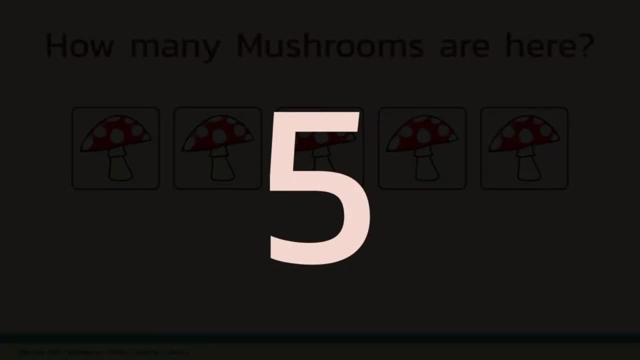 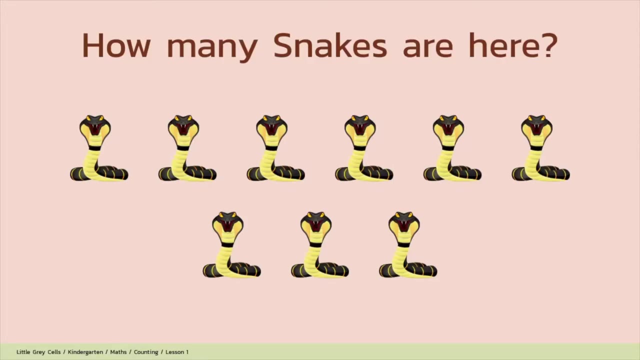 The answer is 5.. Good job, How many snakes are here? All right, shall we count? 1,, 2,, 3,, 4,, 5,, 6,, 7,, 8,, 9,, 10,. 11,, 12,, 13,, 14,, 15,, 16,, 17,, 18,, 19,, 20,, 21,, 22,, 23,, 24,, 25,, 26,, 27,. 28,, 29,, 30,, 31,, 32,, 33,, 34,, 35,, 36,, 37,, 38,, 39,, 40,, 41,, 42,, 43,, 44,. 45,, 46,, 47,, 48,, 49,, 50,, 51,, 52,, 53,, 54,, 55,, 56,, 57,, 58,, 59,, 60,, 51,. 52,, 53,, 54,, 55,, 56,, 57,, 58,, 59,, 60,, 61,, 62,, 63,, 62,, 63,, 64,, 65,, 66,. 67,, 68,, 67,, 68,, 69,, 69,, 70,, 71,, 72,, 73,, 74,, 75,, 76,, 77,, 78,, 79,, 80,. 81,, 82,, 82,, 83,, 84,, 85,, 86,, 87,, 88,, 89,, 90,, 91,, 92,, 93,, 92,, 93,, 94,. 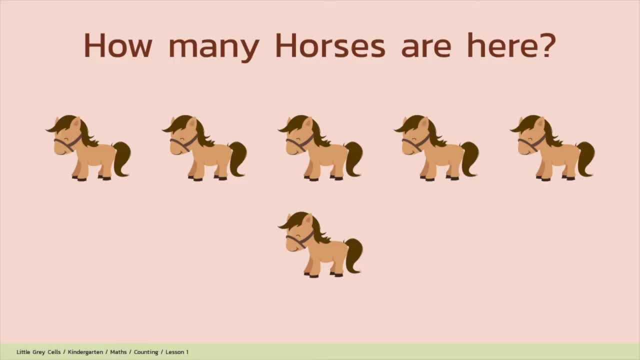 94,, 95,, 96,, 97,, 98,, 99,, 100,, 100,, 12,, 13,, 14,, 15,, 16,, 17,, 18,, 19,, 20,. 21,, 22,, 23,, 24,, 25,, 26,, 27,, 28,, 29,, 30,, 31,, 32,, 33,, 34,, 35,, 36,, 37,. 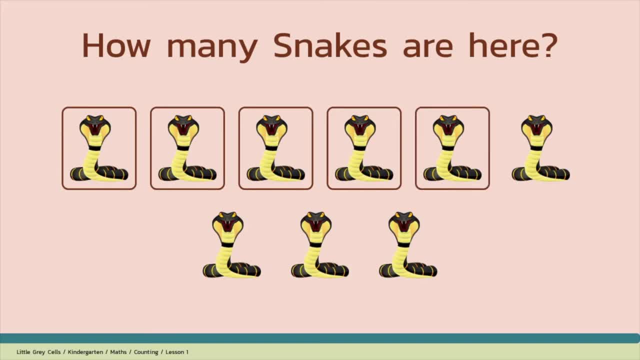 11,, 12,, 13,, 14,, 15,, 16,, 17,, 18,, 19,, 20,, 21,, 22,, 23,, 24,, 25,, 26,, 27,. 28,, 29,, 30,, 31,, 32,, 33,, 34,, 35,, 36,, 37,, 38,, 39,, 40,, 41,, 42,, 43,, 44,. 45,, 46,, 47,, 48,, 49,, 50,, 51,, 52,, 53,, 54,, 55,, 56,, 57,, 58,, 59,, 60,, 51,. 52,, 53,, 54,, 55,, 56,, 57,, 58,, 59,, 60,, 61,, 62,, 63,, 62,, 63,, 64,, 65,, 66,. 67,, 68,, 67,, 68,, 69,, 69,, 70,, 71,, 72,, 73,, 74,, 75,, 76,, 77,, 78,, 79,, 80,. 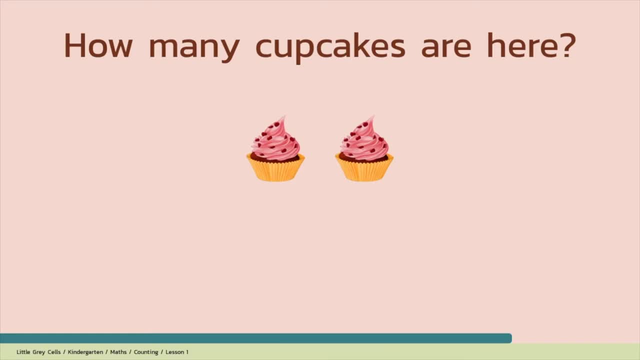 81,, 82,, 82,, 83,, 84,, 85,, 86,, 87,, 88,, 89,, 90,, 91,, 92,, 93,, 92,, 93,, 94,. 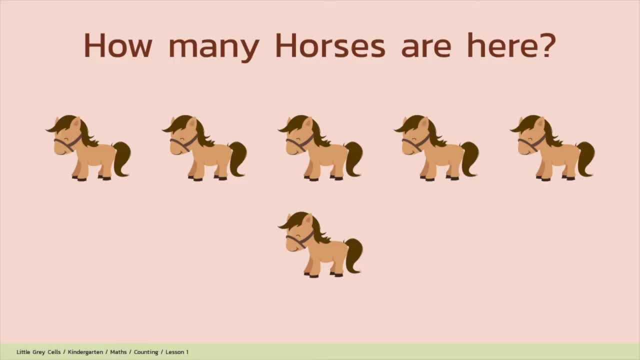 94,, 95,, 96,, 97,, 98,, 99,, 100,, 100,, 102,, 103,, 104,, 105,, 105,, 105,, 106,, 107,, 108,. 109,, 1010,, 1011,, 1012,, 1013,, 1014,, 1015,, 1016,, 1017,, 1018,, 1019,, 1020,, 1021,. 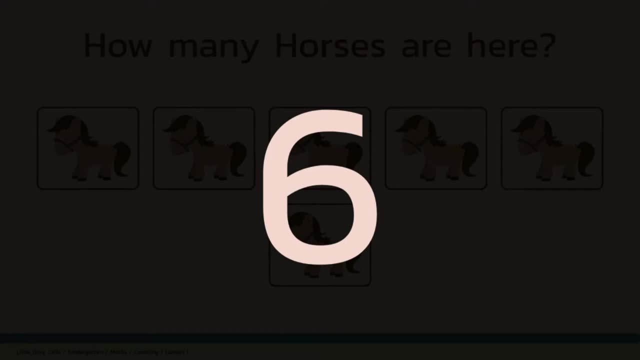 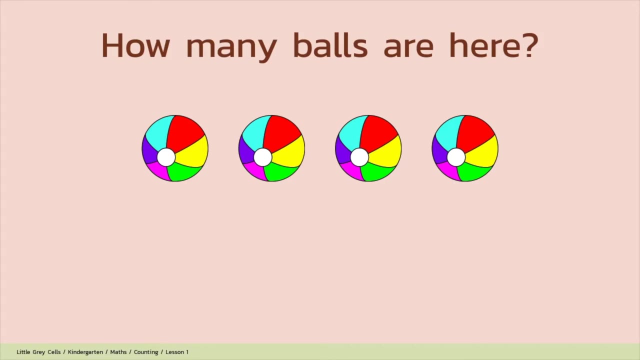 1022,, 1023,, 1024,, 1025,, 1026,, 1027,, 1030,, 1031,, 1032,, 1034,, 1035,, 1036,, 1037,. 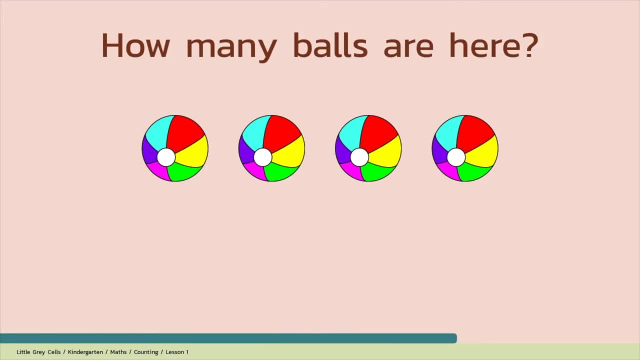 1038,, 1040,, 1041,, 1042,, 1043,, 1045,, 1046,, 1049,, 1050,, 1051,, 1052,, 1053,, 1054,. 1056,, 1057,, 1058,, 1059,, 1060,, 1061,, 1062,, 1063,, 1064,, 1057,, 1069,, 1060,, 1071,. 1072,, 1073,, 1054,, 1062,, 1054,, 1056,, 1069,, 1079,, 1060,, 1070,, 1071,, 1071,, 1062,. 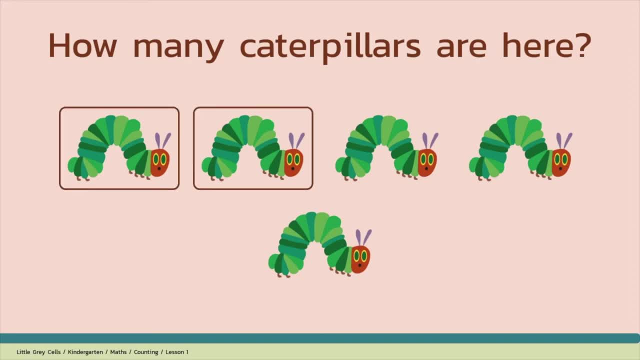 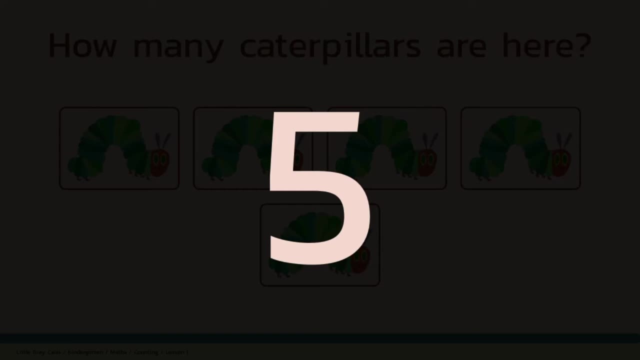 1072,, 1073,, 1064,, 1075,, 1005,, 1006,, 1007,, 1008,, 1009,, 10010,, 10010,, 10011, 5. Good job. 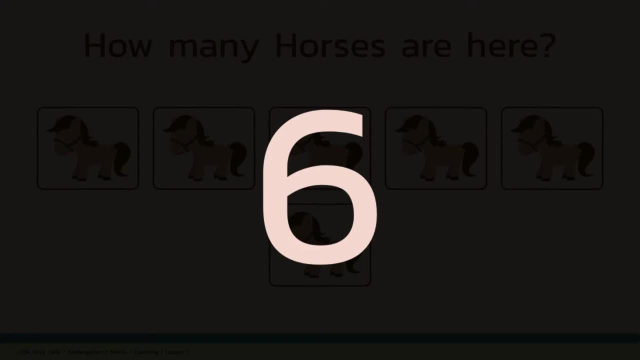 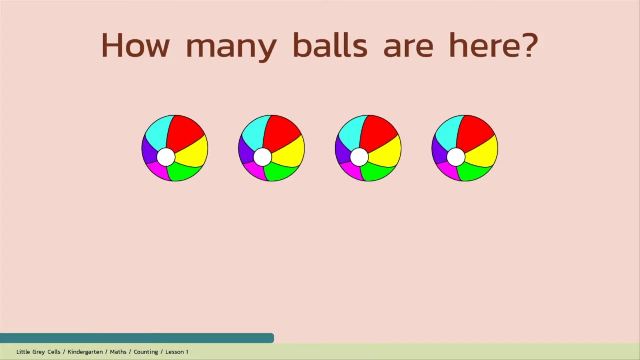 38,, 39,, 40,, 41,, 42,, 43,, 44,, 45,, 46,, 47,, 48,, 49,, 50,, 51,, 52,, 52,, 53,. 54,, 55,, 56,, 57,, 58,, 59,, 60,, 61,, 62,, 63,, 64,, 65,, 67,, 68,, 69,, 70,, 71,. 62,, 63,, 64,, 65,, 66,, 67,, 68,, 69,, 70,, 61,, 62,, 62,, 63,, 63,, 64,, 65,, 65,. 66,, 66,, 67,, 68,, 67,, 68,, 67,, 68,, 69,, 69,, 70,, 62,, 62,, 65,, 62,, 63,, 62,. 65,, 62,, 33,, 33,, 34,, 34,, 35,, 35,, 36,, 36,, 37,, 37,, 38,, 39,, 40,, 60,, 60,. 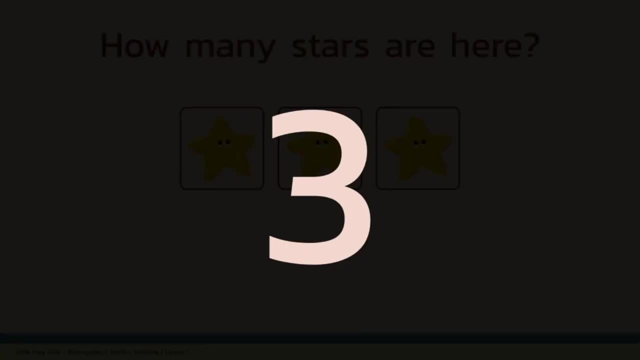 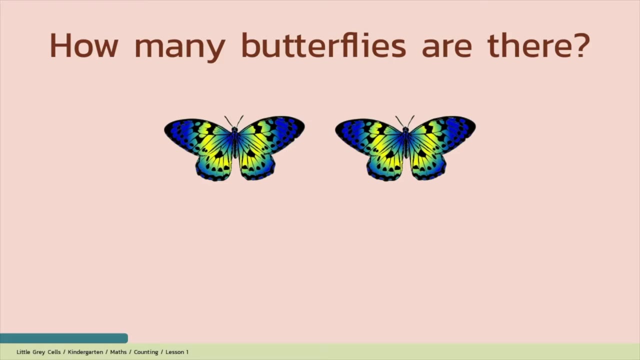 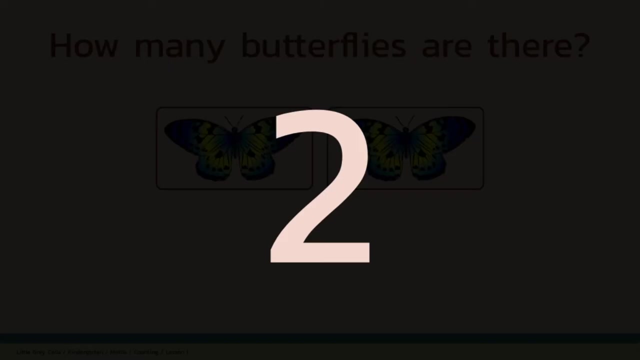 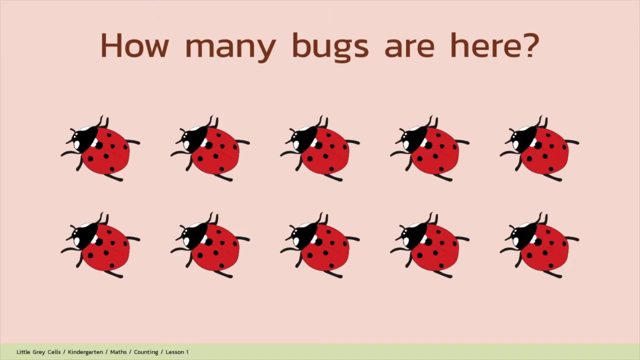 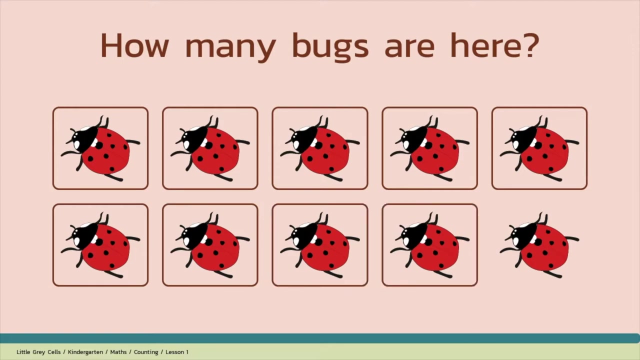 70,, 70,, 81,, 81,, 80,. how many butterflies are there, all right? shall we count one, two? the answer is two, good job. how many bugs are here, all right? shall we count one, two, three, three, four, five, six, seven, eight, nine, ten? the answer is ten, good job. 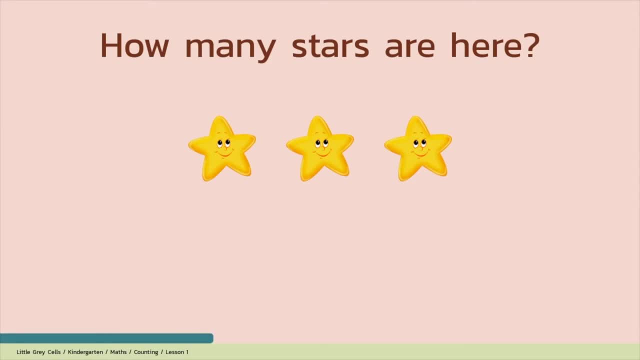 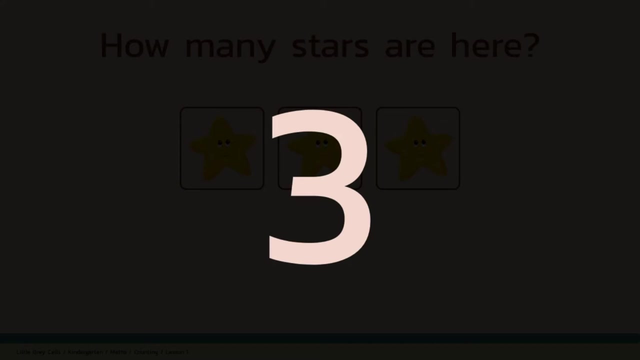 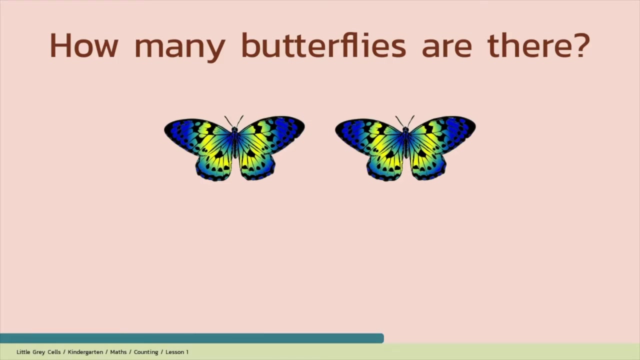 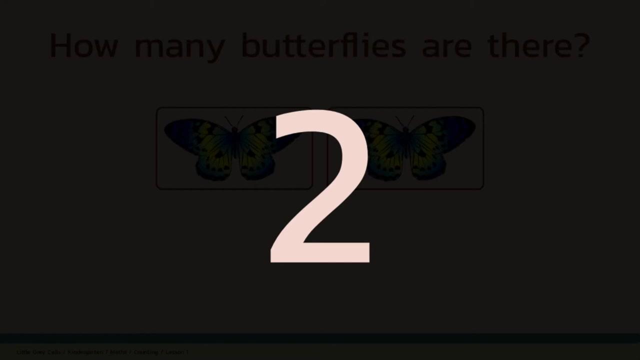 How many stars are here? Alright, shall we count 1, 2, 3? The answer is 3. Good job. How many butterflies are there? Alright, shall we count 1, 2? The answer is 2. Good job. 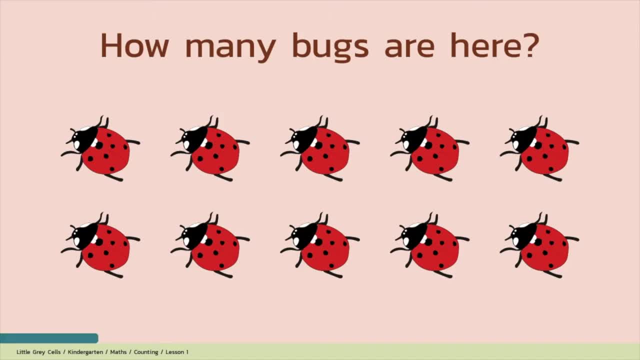 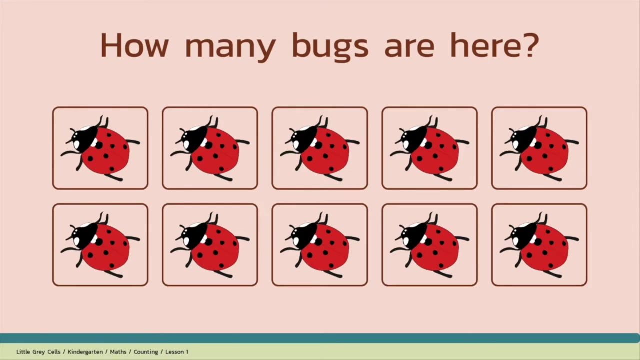 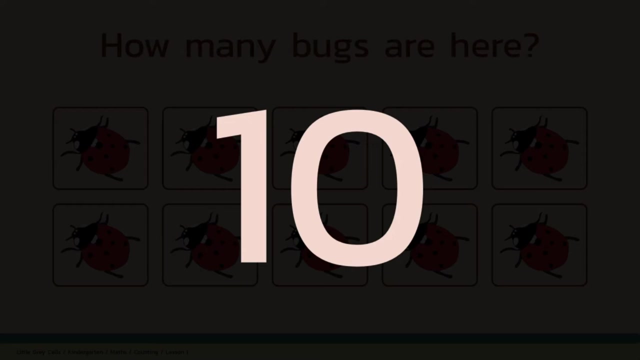 How many bugs are here? Alright, shall we count? 1, 2, 3, 4, 5, 6, 7, 8, 9, 10. The answer is 10.. Good job, How many girls are here? 1, 2. 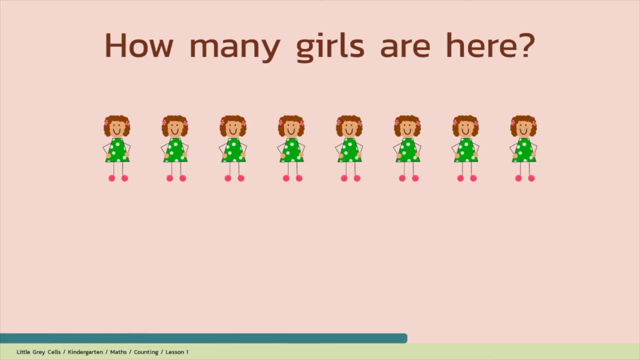 3, 4, 5, 6, 7, 8, 9, 10, 11, 12, 13, 13, 14, 15, 16, 17, 18, 19, 20, 21, 22, 23, 24, 25, 26, 27. 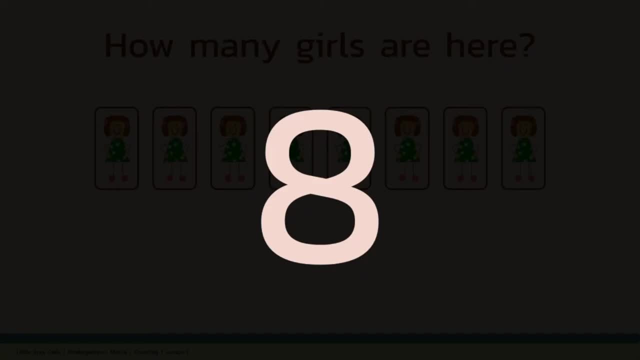 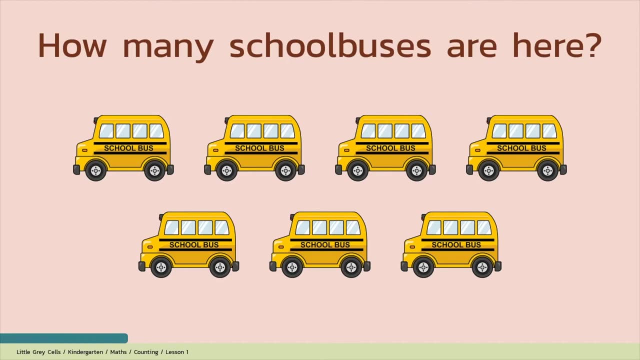 28, 29, 30, 31, 32, 33, 33, 33, 34, 35, 36, 37, 38, 39, 40, 41, 42, 43, 44, 45, 46, 47, 48, 49, 50, 51. 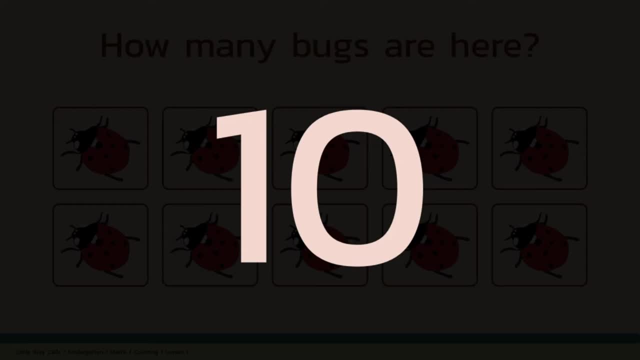 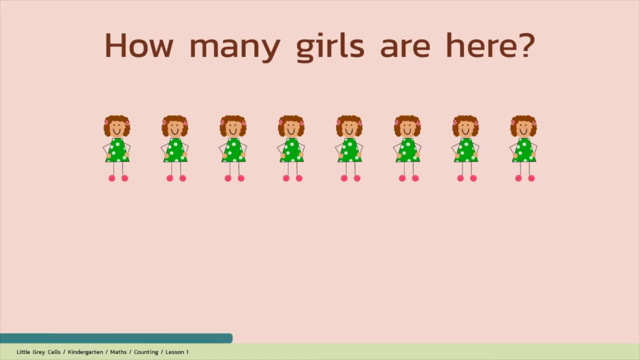 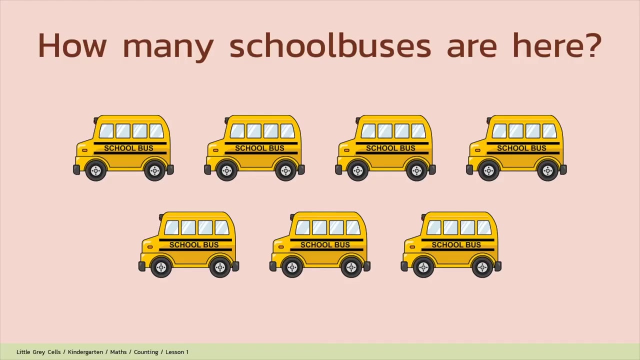 how many girls are here? all right. shall we count one, two, three, four, five, six, seven, eight? the answer is eight, good job. how many school buses are here? all right. shall we count one, two, three, four, five, six, seven, eight? the answer is all right. shall we count one, two, three, four, five, six, seven, eight? the answer is: 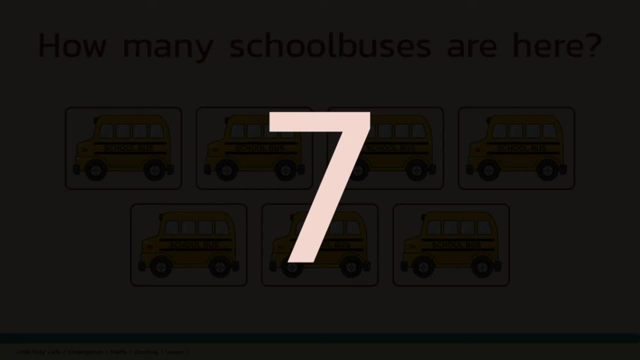 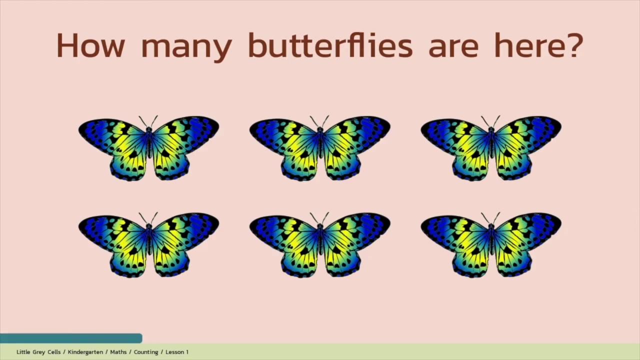 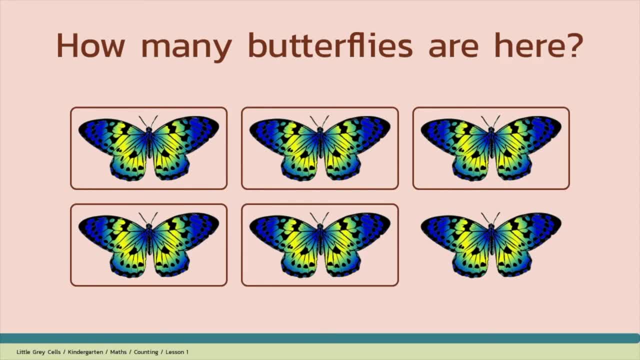 all right. shall we count one, two, three, four, five, six, seven, eight? the answer is seven. good job three, four, all right. shall we count one, two, three, four, five, six, seven, eight? the answer is seven, good job three, all right. shall we count one, two, three, four, five, six, seven, eight? the answer is seven, good job three. 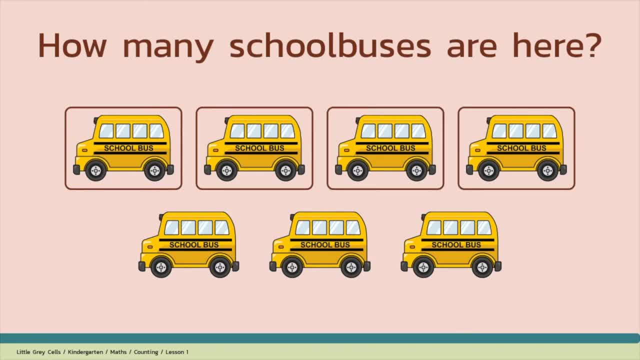 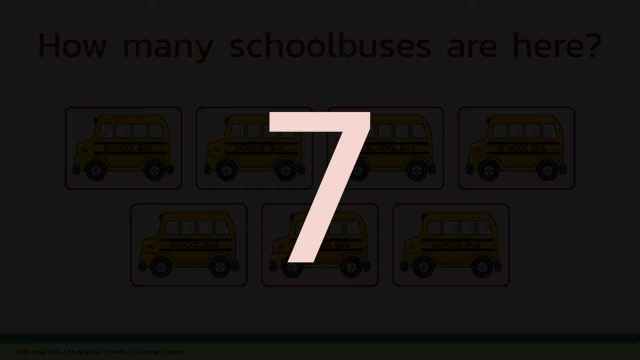 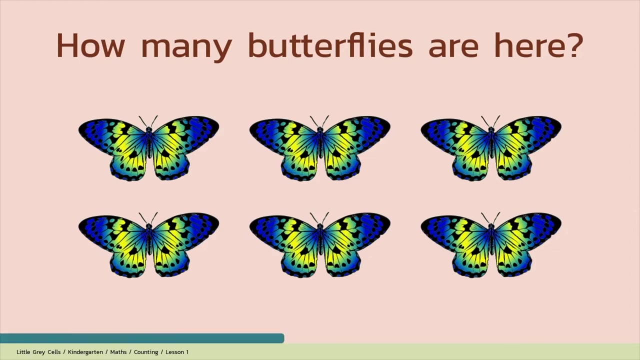 52, 53, 54, 55, 56, 57, 58, 59, 60, 60, 61, 62, 63, 64, 65, 66, 67, 68, 69, 70, 71, 72, 73, 74, 75, 76. 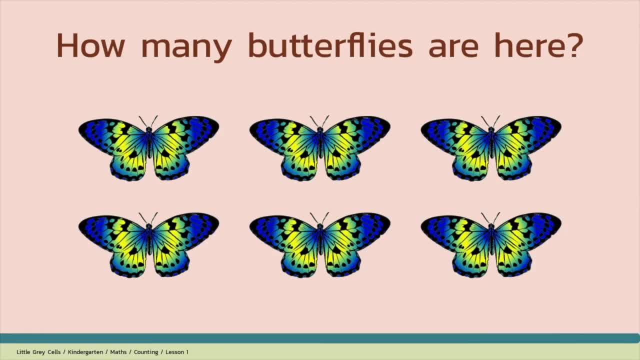 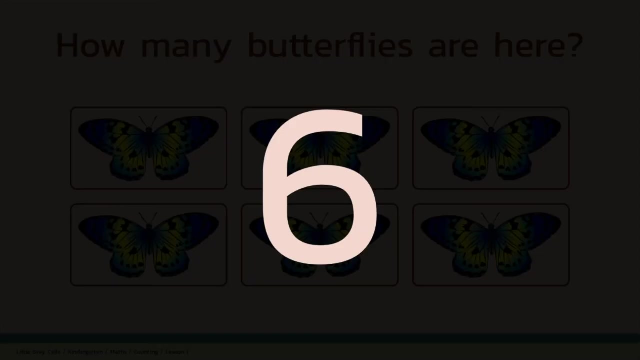 76, 77, 78, 79, 80, 81, 82, 83, 83, 84, 85, 86, 87, 84, 85, 86, 87, 88, 89, 90, 91, 92, 93, 93, 94, 95. 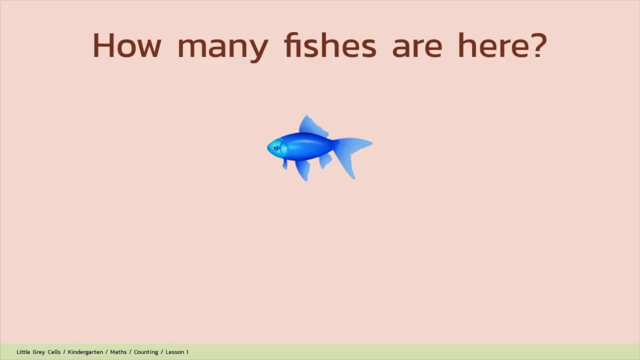 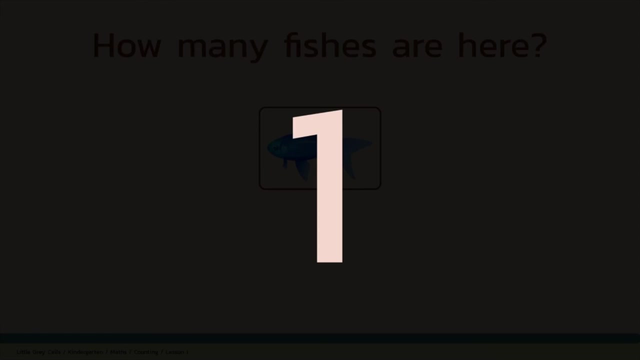 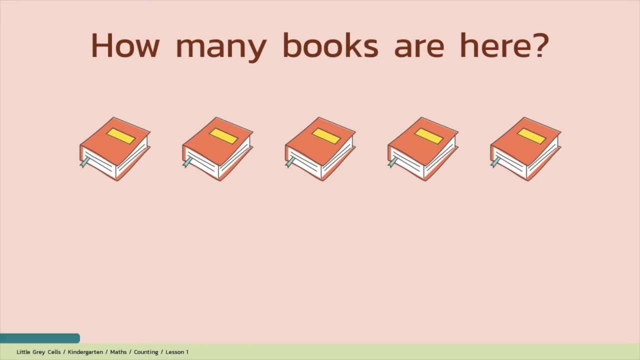 96, 97, 98, 99, 100, 10, 11, 12, 13, 14, 15, 16, 17, 18, 19, 20, 22, 23, 24, 25, 26, 27, 28, 29, 30, 31. 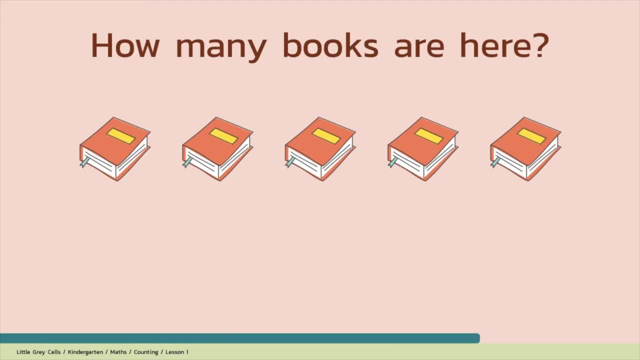 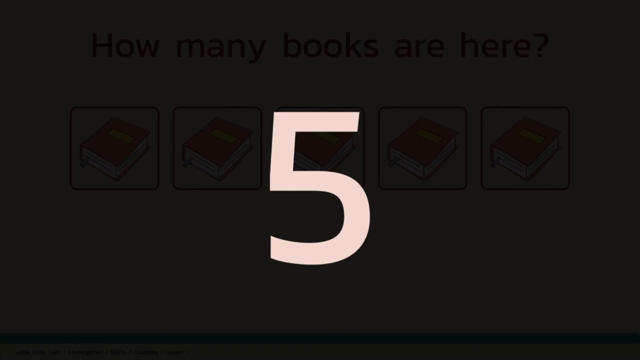 32, 33, 34, 35, 36, 37, 38, 38, 39, 40, 41, 42, 43, 44, 45, 46, 47, 48, 49, 51, 52, 53, 52, 53, 54, 56. 57, 58, 59, 60, 61, 62, 63, 64, 65, 66, 67, 68, 69, 69, 70, 71, 72, 73, 73, 74, 74, 75, 75, 76, 74, 75. 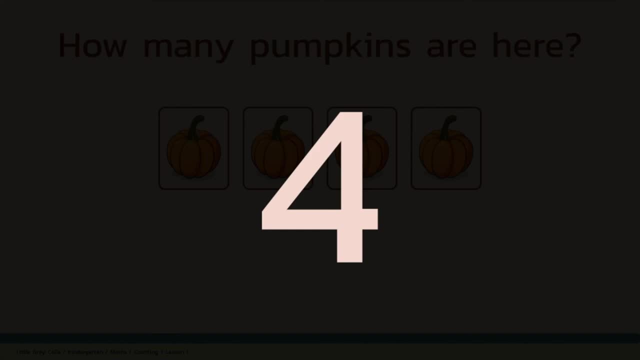 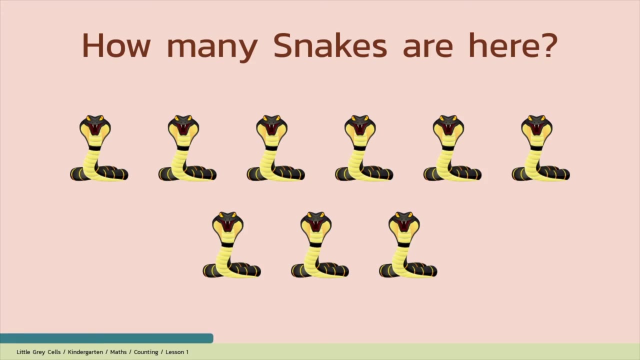 76, 77, 78, 78, 79, 80, 81, 82, 83, 84, 85, 86, 87, 88, 89, 90, 91, 92, 93, 93, 94, 95, 96, 97, 97, 98. 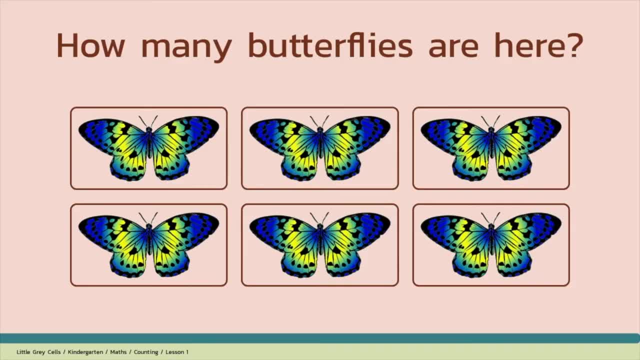 all right. shall we count one, two, three, four, five, six, seven, eight? the answer is seven, good job. three, all right. shall we count one, two, three, four, five, six, seven, eight? the answer is seven, good job. three, all right. shall we count one, two, three, four, five, six, seven, eight? the answer is seven, good job. three, six, good job. 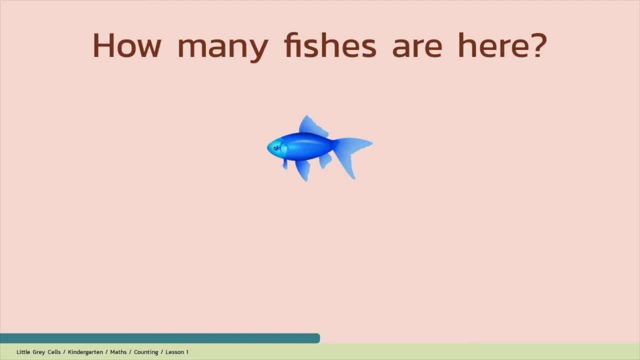 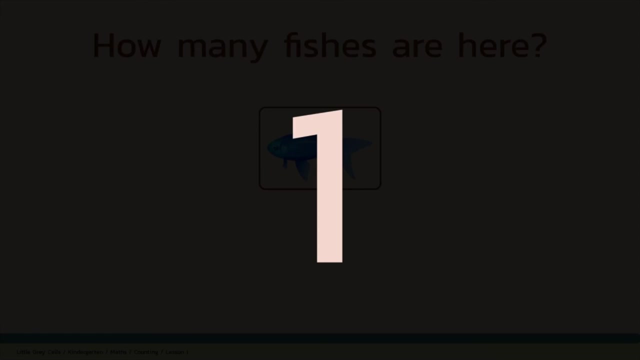 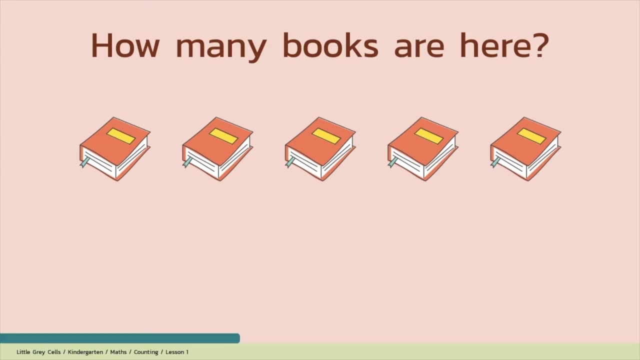 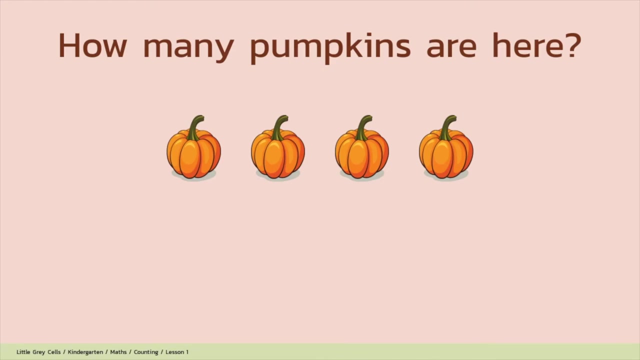 how many fishes are here? all right. shall we count one? the answer is one, good job. how many books are here? how many pumpkins are here? all right. shall we count one? all right. shall we count one, two, three, four, five? the answer is five, good job. how many pumpkins are here? 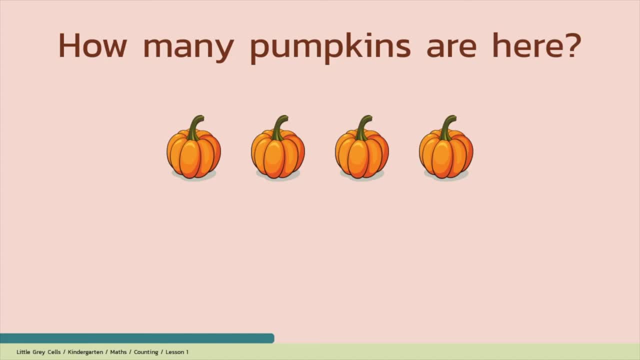 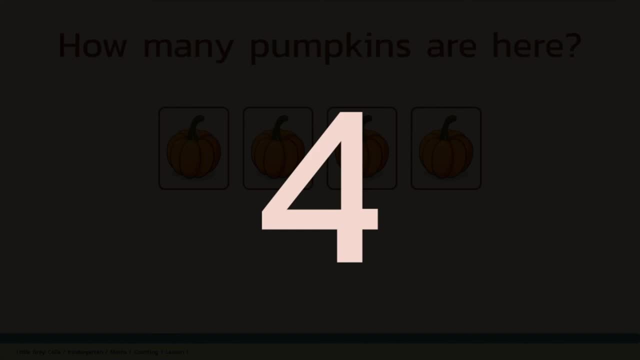 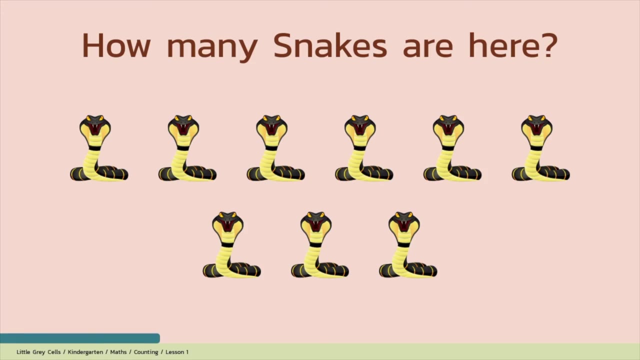 the answer is four. good job, how many snakes are here? how many snakes are here? how many snakes are here? all right, shall we count one, two, three, four, five, six, seven, eight? the answer is seven. good job, all right. shall we count one, two, three, four, five, six, seven, eight, nine? 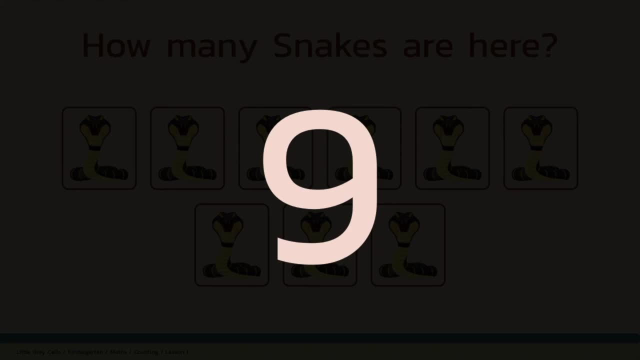 all right. shall we count one, two, three, four, five, six, seven, eight, nine? the answer is. the answer is: the answer is nine. good job. if you like this video, please share with. if you like this video, please share with. if you like this video, please share with your friends. 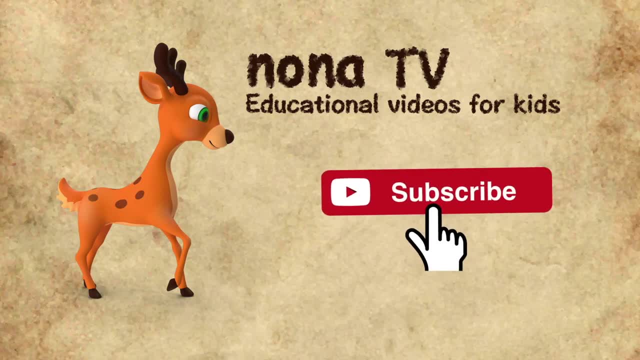 your friends, your friends, and don't forget to subscribe for more. and don't forget to subscribe for more. and don't forget to subscribe for more. educational videos. educational videos.